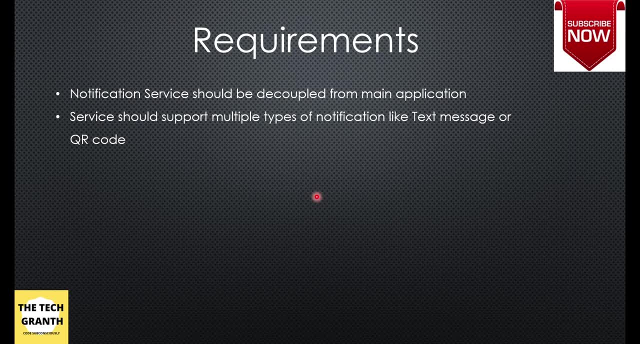 notification, you should be able to send a text message or a QR code or, in future, you should be able to send any other form of message. next is that the service should support multiple types of sending and multiple ways of sending your notification, so you should be able to send your notification as a text which. 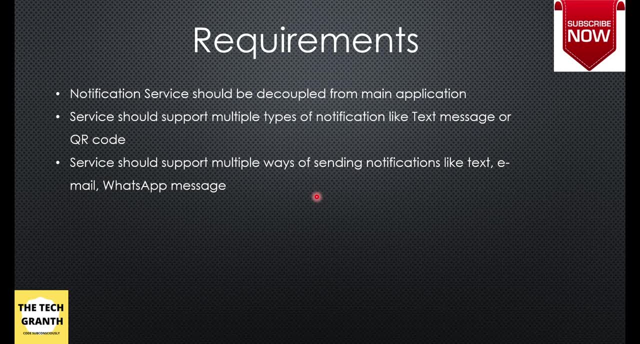 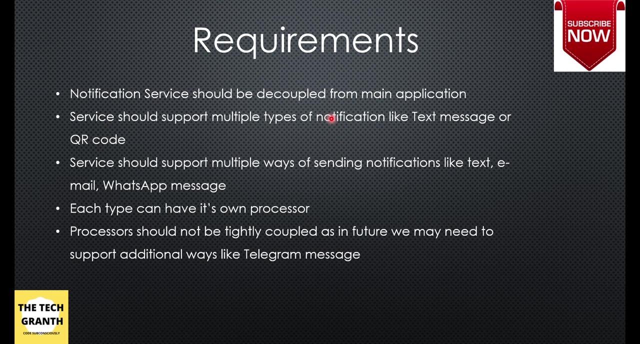 will be an SMS or an email or whatsapp message, and each type that you have it can have its own processor. so so that they all have their own single responsibility. and finally, the processor should not be tightly coupled, because in future we may want to basically add the new way of sending notification, like we want to send a. 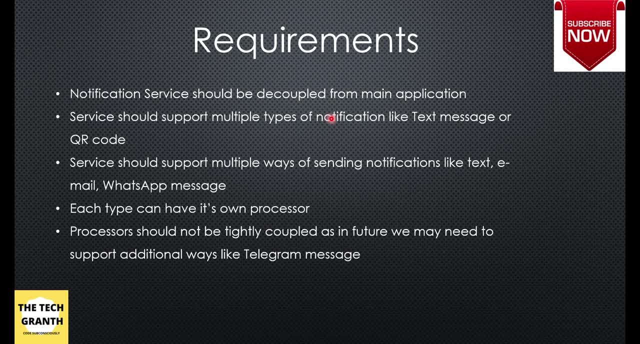 telegram message rather than whatsapp message, or we even want to add a new type of message, so that suppose it's like if it is an internal application. so rather than a text message, i want to send a JSON or an XML message. that kind of scenario can come. so you should be able to handle, or your application should be able to handle. 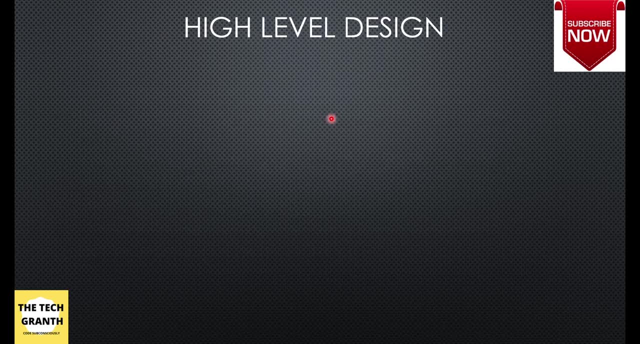 that kind of scenario. so the high-level design for this will look something like this: where we will have some external application which wants to send a notification, we will have a queue. so whatever notification that the application wants to send, its can put it in a queue and from queue we can pick up that particular application. so we will have a. 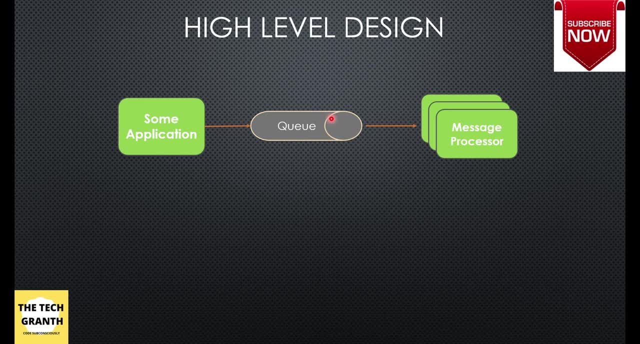 message processor on our side which will pick up that particular message that has to be sent and it will process that. so what message processor will do is it will read the notification coming from the application so that it identifies. so this can be in a json format or an xml format. 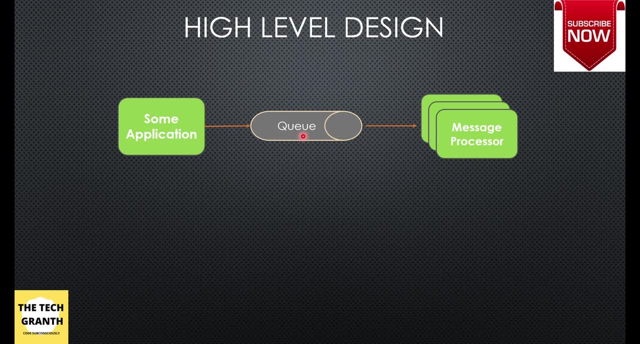 and it can have multiple tag which will tell us that, okay, this message is of type text message or a qr code, and i want to send this message as a whatsapp message or email or maybe sms. so all those things can be added as part of the json format which this application can send it into. 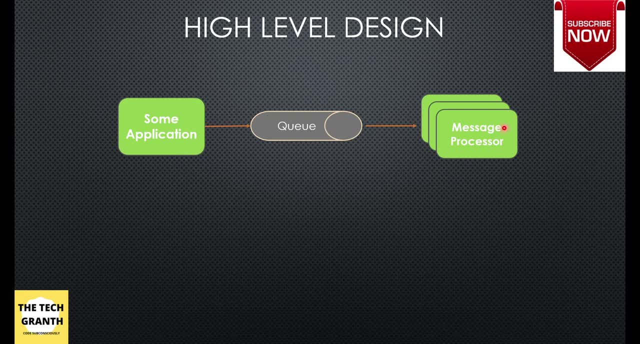 the queue, so that can be a contract between the application and the message processor. these can be customized. and finally, some design consideration. so we should have a scale, we should have this application so that the service can scale in case the there are a lot of traffic on the application, so you should be able to scale. 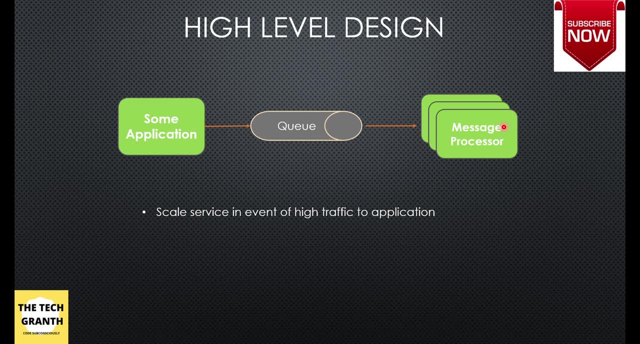 the application in the event when there is a lot of traffic on your application. for example, when you are booking using a system like book my show on fridays or weekends, you will get a lot of ticket booking, so you should be able to handle that so that you can send the notification. or 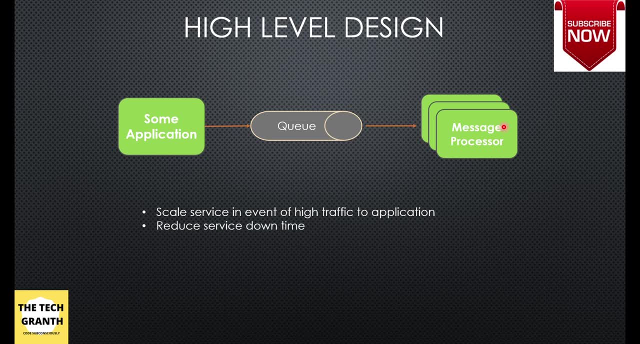 the tickets to all the person who have booked the ticket. you should reduce the service downtime so you know that you can send the notification to all the person who have booked. the ticket notification service should be really reliable and it should be down for minimum time so that the 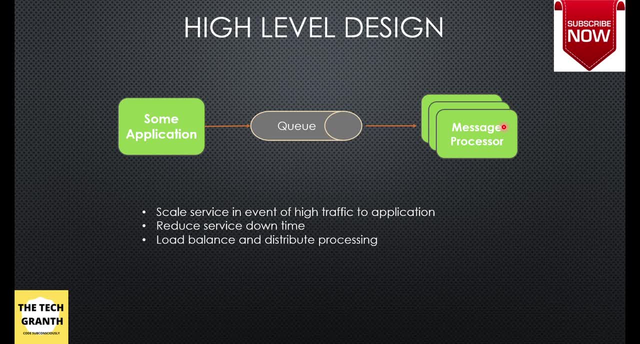 tickets can be sent as soon as possible. and, finally, you should be able to load, balance and distribute the processing. so the idea here is that you should come up with a microservice architecture and you should be able to scale it up. so if you want to learn about how you can scale your 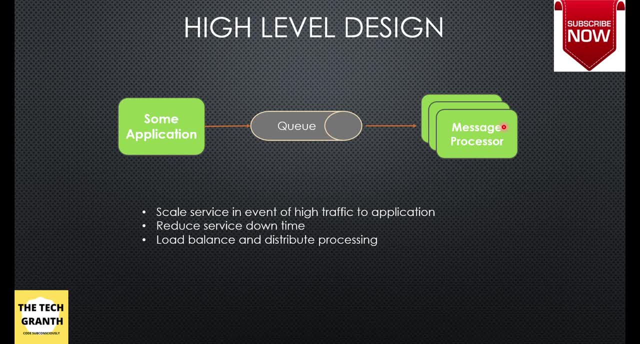 microservice architecture, what design pattern you use for that. you can watch my video- the link is there in the description- and there is a playlist for microservice architecture tutorial which i have created sometime back so you can have a look at that also. so this is the overall high level design for the notification service. we'll jump into message. 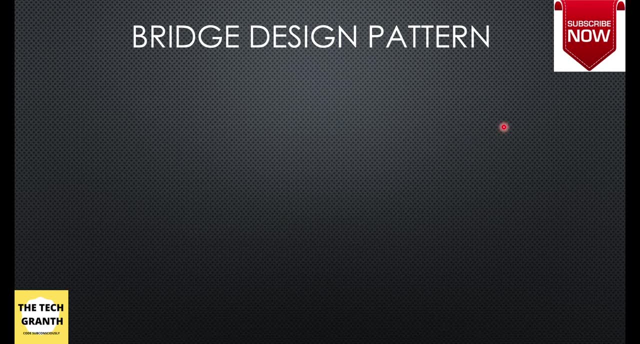 processor and we'll talk in detail about it. so the message processor that we are going to build will be based on bridge design pattern and we'll see why it will be based on bridge design pattern. so before talking about that, let us understand what a bridge design pattern is. so what bridge? 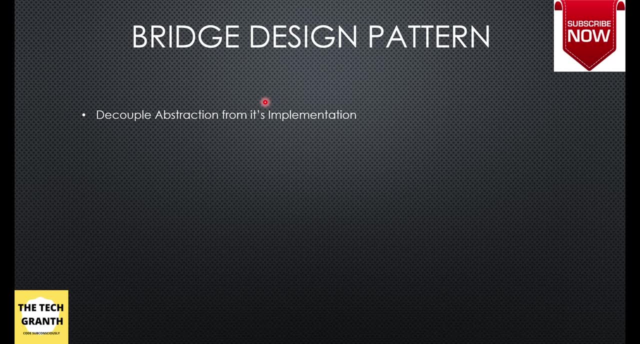 design pattern does is it decouples the abstraction from its implementation. so there is a set of abstraction and there is set of implementation. so what it means is you define something and then you implement that something. so these two should be separate from each other. that is what the bridge 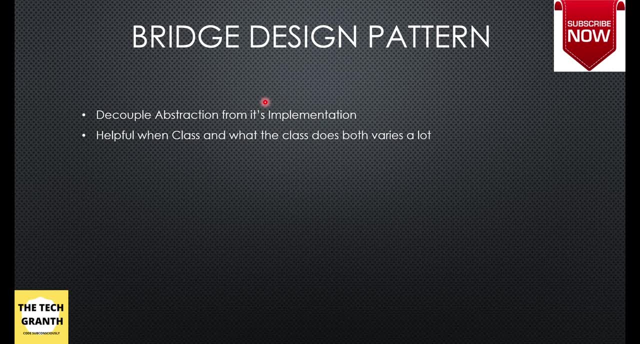 design pattern tells us. now it is helpful when the component, which is your class, and the method what? what it means? is that what the class is going to do? so there are two things: there is a template, which is your class, and there is the action that will be taken by the class. both will vary and 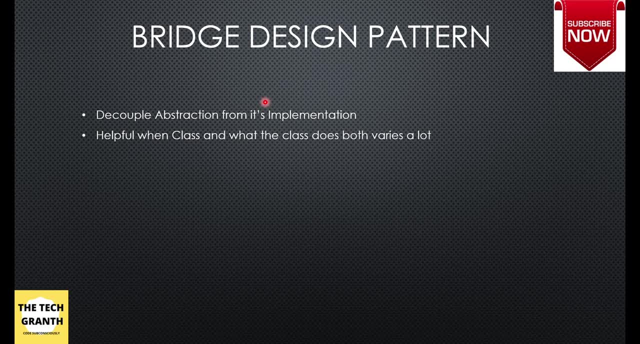 both can vary a lot. for example, in our case, we have a template which is messaging or the notification that we are going to send, so we have different notification that we support like text message, qr code, maybe json, xml, anything. so we have different notifications that we support like text message, qr code, maybe json, xml, anything. 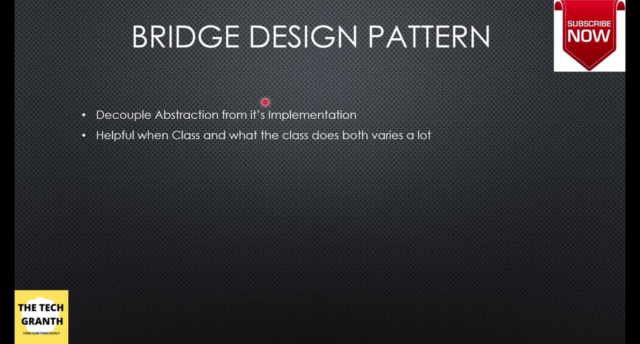 like that and we have a way to send these message or send these notification, which will be via sms, email or whatsapp message, maybe telegram message. so there are two things here: there is a template, which is the message type or the notification type, and there is the implementation, where we are. 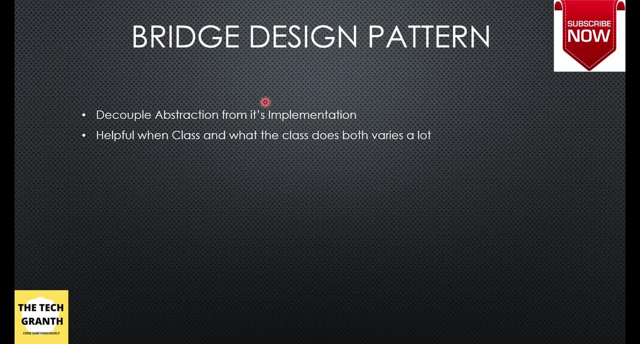 there are ways in which we can send that particular message, so these are two different thing. one is the abstraction, other is the implementation. like i said, in our case, notification can be text, email, whatsapp, and the way you send- is you send a text message or sms email, whatsapp? 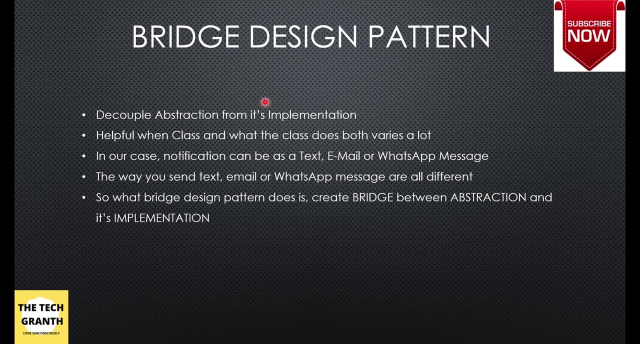 message. all are different, so what bridge pattern will do here is it will create a bridge between the abstraction and its implementation, so don't worry about it. if you are not able to grasp it straight away, just pause the video, go back and watch it again and, going further, i will code for. 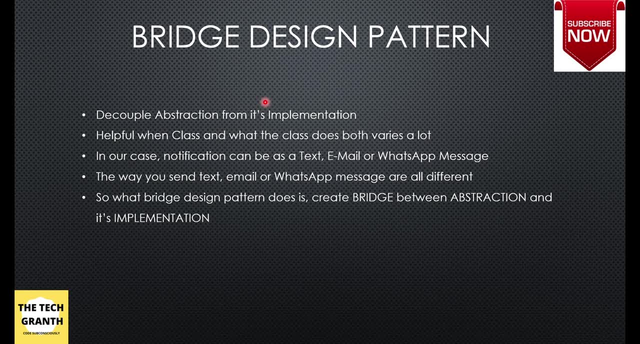 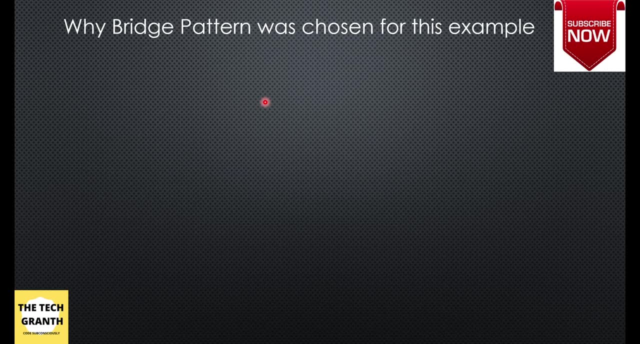 it. so it will be little more clear that how you can apply this bridge pattern and what is the abstraction part, what is the implementation part, so why we have chosen bridge design pattern for this particular example. so some, a lot of people have asked a question that how we will decide that which pattern to 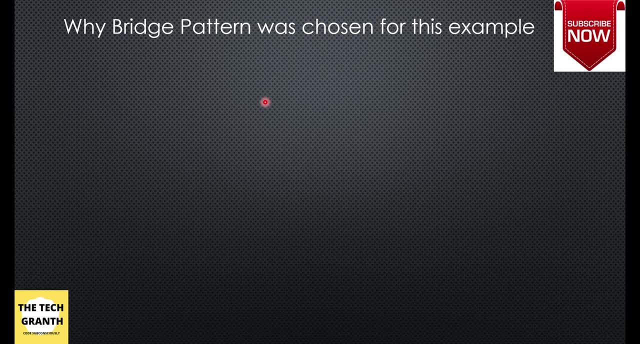 use in a particular case, because some of the pattern look very close. i will create a separate video for that, where i can compare the various pattern and i'll come up with the solution: that in which scenario we should use which design pattern, but in this pattern, in this particular case, the question is why bridge pattern was chosen in this example. so first thing, 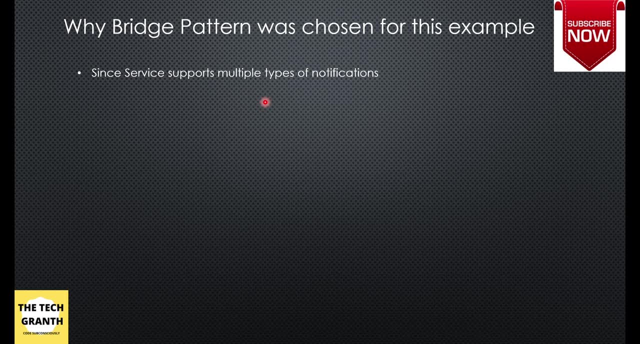 is that, since the service support multiple type of notification, multiple type of notifications are there, which we can think of as an abstraction for sending the messages, and each type can be implemented in multiple ways based on where we need to send the message. so there is a template. 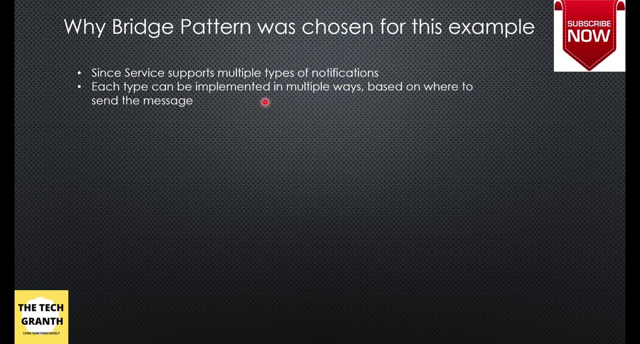 for notification and there is a way to send the notification. so there are two things. so consider an example: if you want to send the message, you want to type ua before it starts. so this is the same information, starting from three relationship up to one, and in the next is what will be know, and that is the 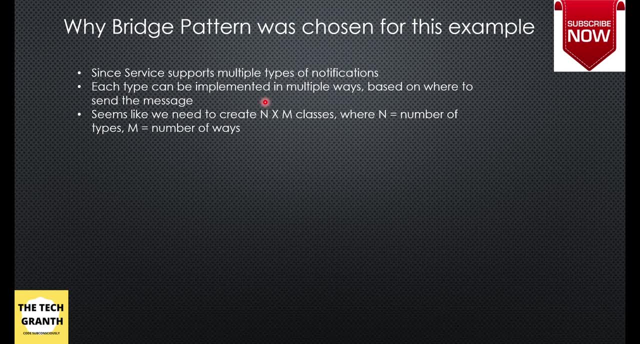 initial result, and it was. it starts a model of the pre-action which is trying to into 거죠 because does this work? i will use this model, which is trying to add a reason to the model, to the model you see here. here is the result. 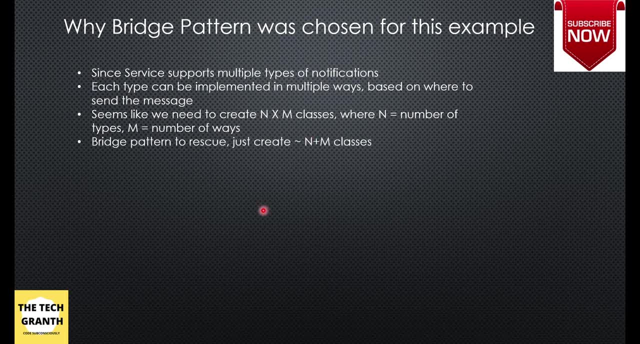 which is 6, but if we use bridge design pattern, so in this particular case we will end up creating n plus m classes, which will be number of types and number of ways of sending the message. so as the number of type and ways increases, you can understand that it will be growing in that. 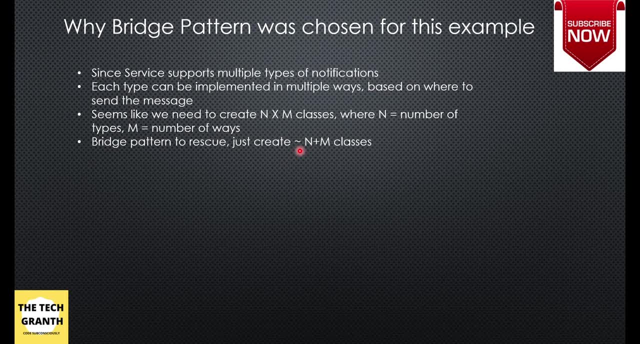 particular way and why it says that it's almost equal to n plus m, the reason being that you will create a couple of class for your to implement your pattern. basically, you will create some interface and abstract class for that. that is why it's almost equal to n plus m, now the abstraction. 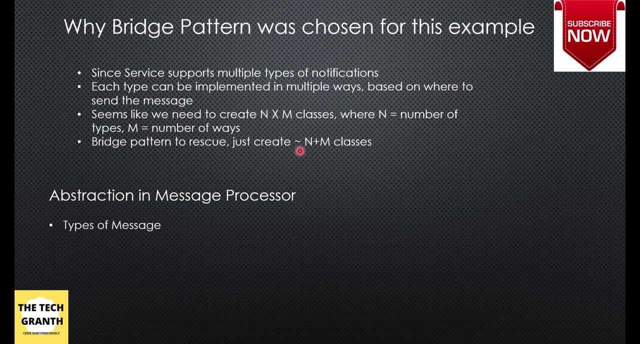 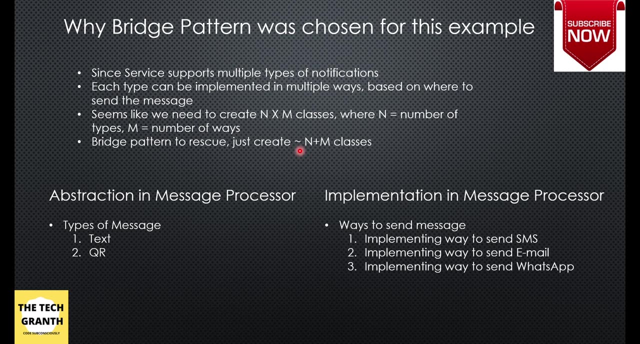 that we were talking about as part of this message processor was we have types of message, which is text and qr code, and the implementation that we talked about is the way to send the message. so we are implementing the way to send sms, implementing the way to send email and whatsapp. so this part- 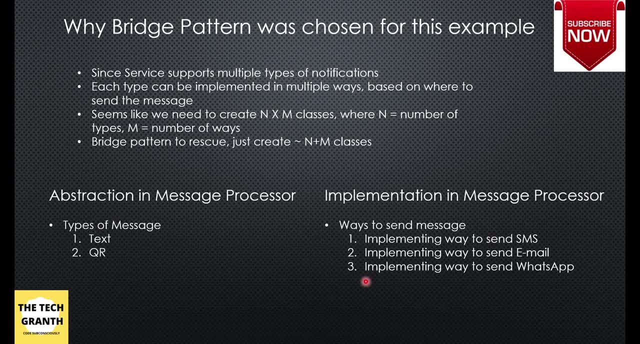 is the n part, this part is the m part. so the bridge pattern is the way to send the message. so the bridge pattern, what it will do is it will create a bridge between these two and it will make our life easy to create this notification service. now next thing is that we'll jump into the code. 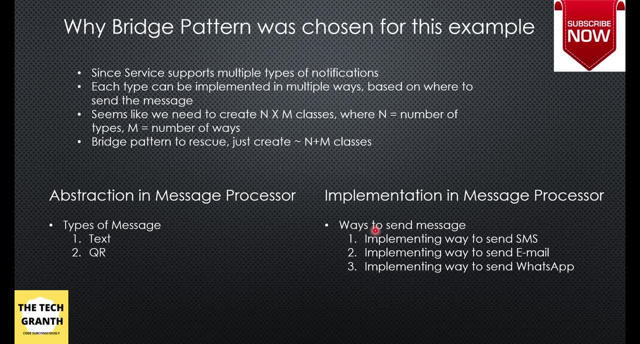 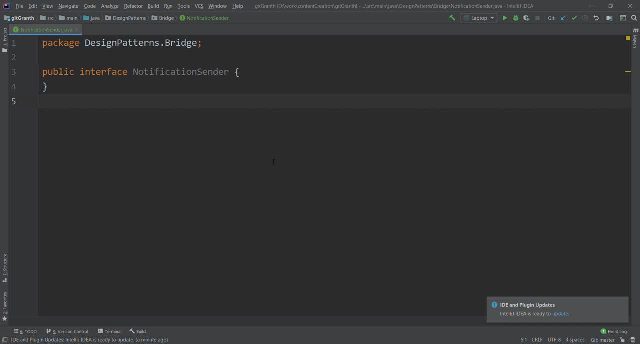 and we'll see how we can implement the bridge pattern to come up with the notification service. so to implement the bridge pattern, first we will create a notification sender, so this will lie on the implemented implementer side. so, like i explained, for the bridge pattern there are two. 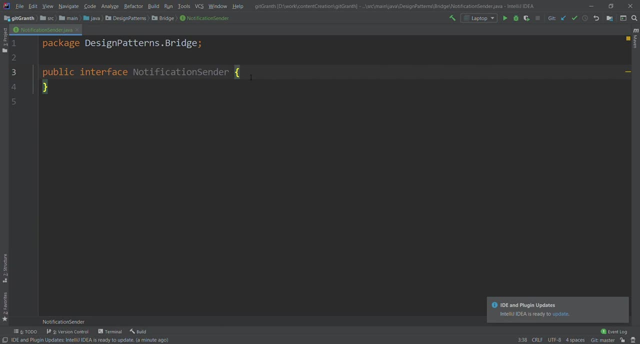 parts abstraction and the implementation. so what notification sender will do is it will be an interface and it will have a method: send notification. so any any sender that we are going to implement, they will basically, uh, implement this particular interface and creates its own way to send the notification. so we have this and now we have to. 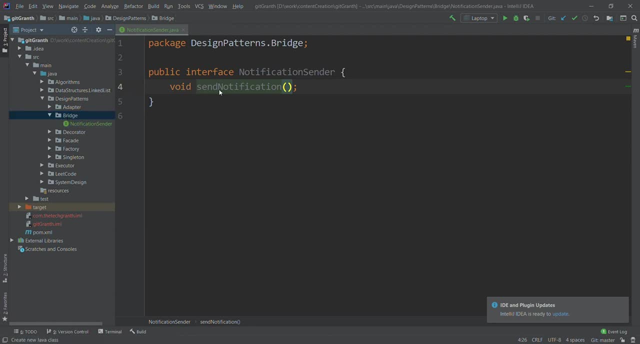 create an abstraction. so we need to create an abstract class, which will be an abstract class, which will be an abstraction of the types of notification that we need to send. so we'll call it notification. let us say let's call it notification and we'll create it as an abstract class. 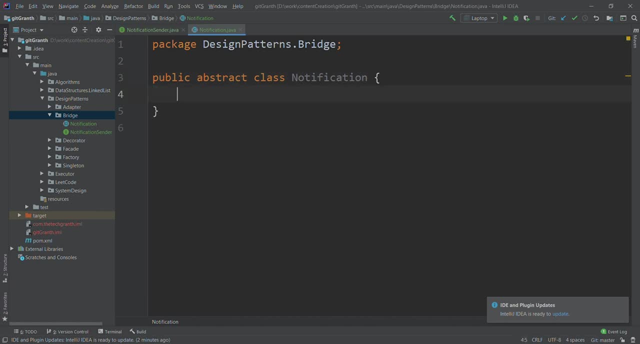 so this will have the, this will have the notification sender- whatever notification sender that we have- and let us add it in the constructor, or to insert. this will be added in the constructor and each message will have its own type of method which will be sending the notification. so the- basically notification has to be created and 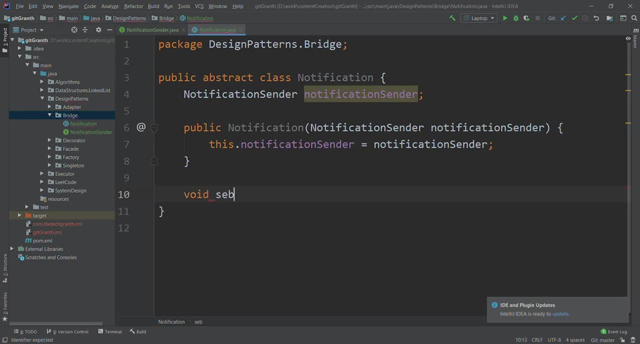 sent, so this will be void. send message or send notification. we already have a notification sender here which we send that send notification, so let us call it send message. it does not matter, we could have named it same, and this will be abstract method. let us now have all our abstractions first. so the first abstraction that we will have is text message. 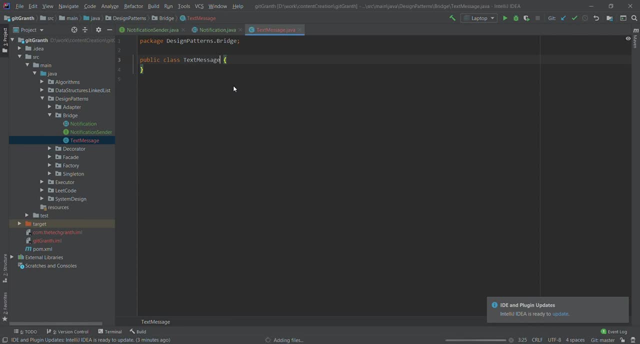 so this can extend the notification class and once we have the notification class, this would be able to send the message and we can basically add the constructor here. so this will call the super and here we will have this dot: send notification. so this will be able to send the message and we can basically add the constructor here. 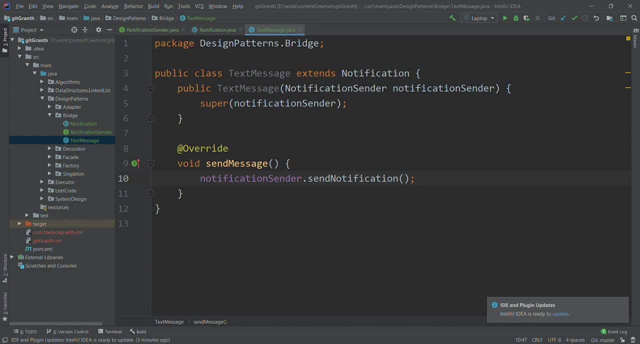 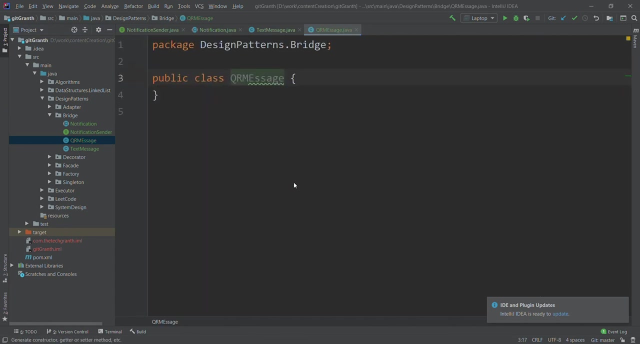 so this will send notification for any text base notification. so if there is a notification which will send a text message, this, that type of that type of message, will be handled by this particular class. let us create one more. so here we will have the qr message. let me refactor this. 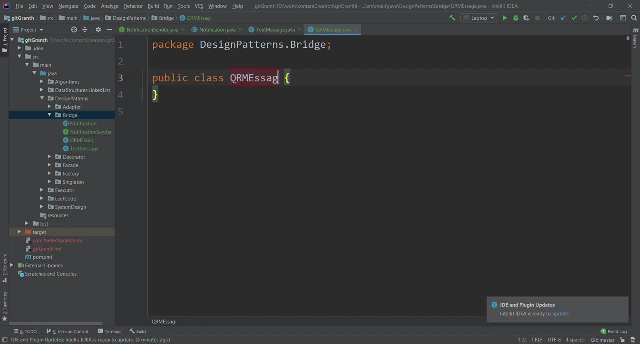 qr a message, and this will again extend the notification class we had. so we'll implement this method and we'll add the constructor also. so this is here and we'll have notification sender dot, send notification. so what this will do is in send message we can build some additional message which will be for qr code. here we can call: 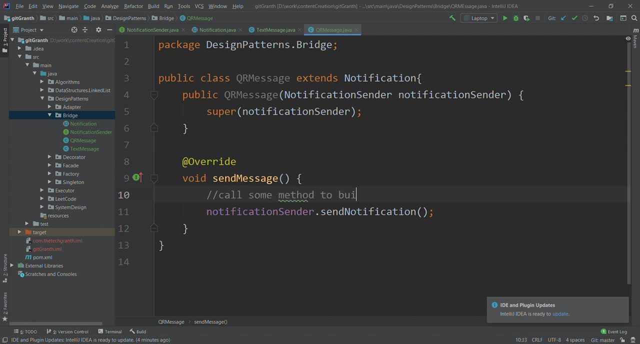 call some method to build qr code so you can add something here and finally, you send the message. so you use this send message to send the send notification via some channel. now that channel will be based on whatever is added as part of this constructors, whatever been you invoke using this constructor. now these two. 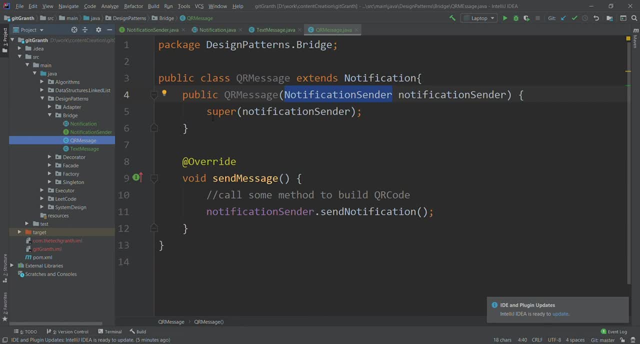 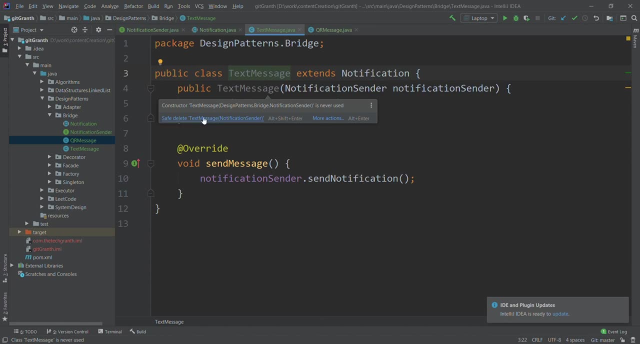 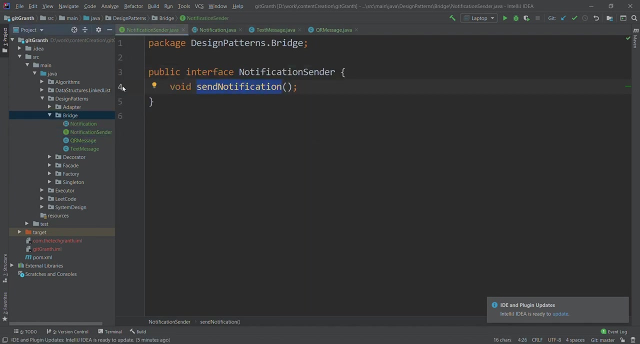 classes: the QR message and the text message. these two classes are basically the abstraction part, which define the type of notification we are going to send. the second part was the implementation, for which we created this notification sender. so let us create the implement concrete implementation of the this implementer. so first one will be sms. let us call the class as sms itself and this will implement the notification sender. 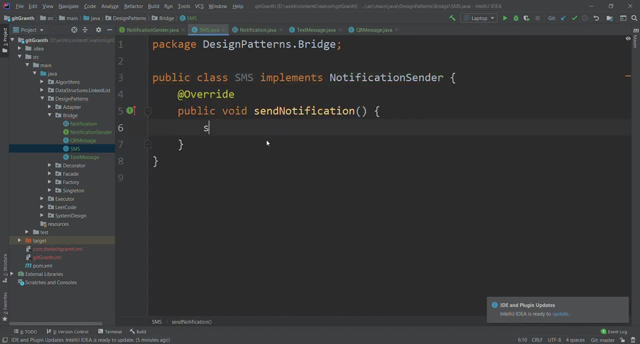 and here we can say: system dot out, we are going to send sms. similar to this: we can click create another implementation which will be for email. this will implement again the notification sender and here we can say out sending an email, okay. and for for text message and all we. 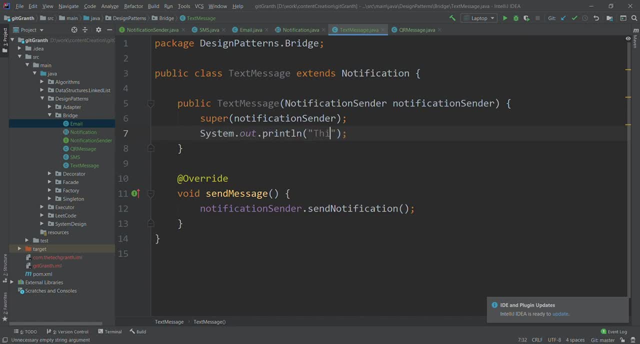 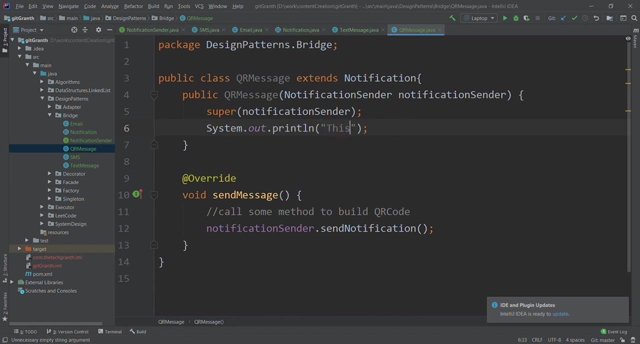 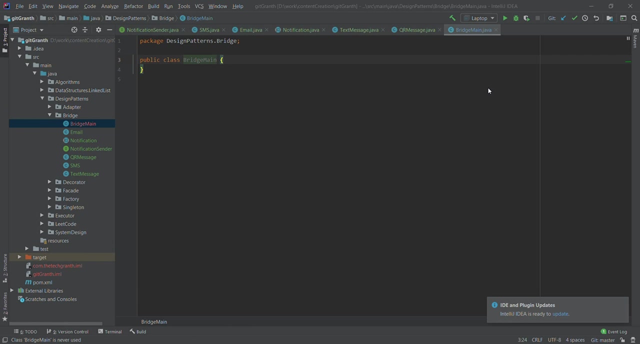 can add a simple shout here saying that this is a text message and the other one was the QR message. so here we can add: this is the QR code. let us create a bridge implementation or the main class. let's call it bridge main, so this will have public static void mean here and here. we will now suppose we want. 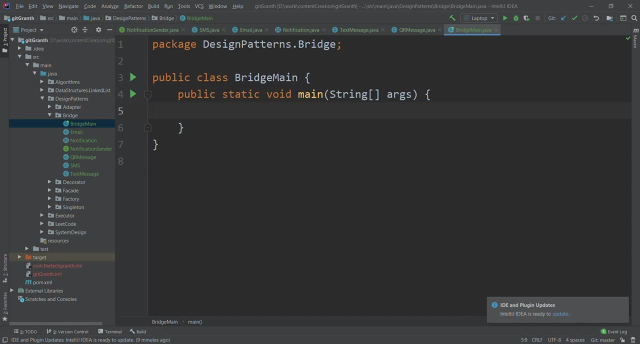 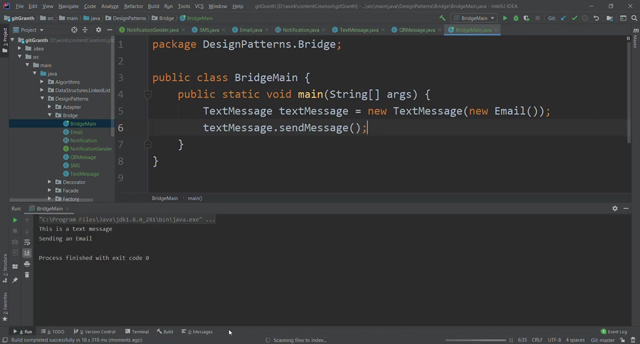 to send a text message over, let's say, email. so what we'll do is we will create text message equals to new text message and this will have email, and we'll have text message dot send message. let us run this. it takes a second to compile, so it says that this is a text message sending an email. so this was sent via an email. now. 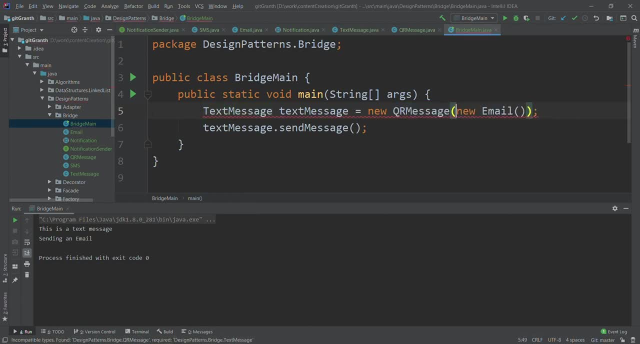 suppose this was qr message and this will be qr message. this will be qr message and i want to send it. okay, we'll send it as email first and then we'll send it as sms. so it says that this is qr code- sending an email- and if we use sms, so this will do the same. 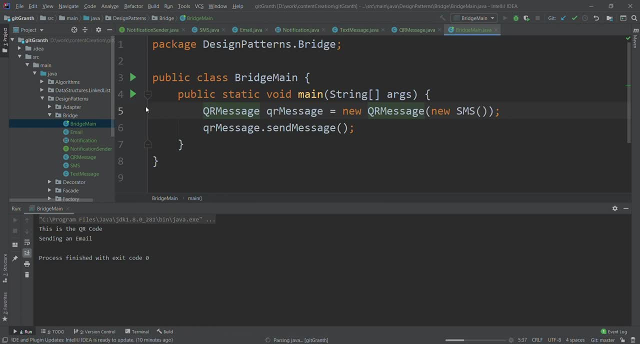 thing: it will create the qr code and it will send it as an sms. so we are going to send sms. so here we saw that when we have a situation where we have to create n, cross, m kind of class, we'll use bridge pattern to separate the abstraction from the implementation. 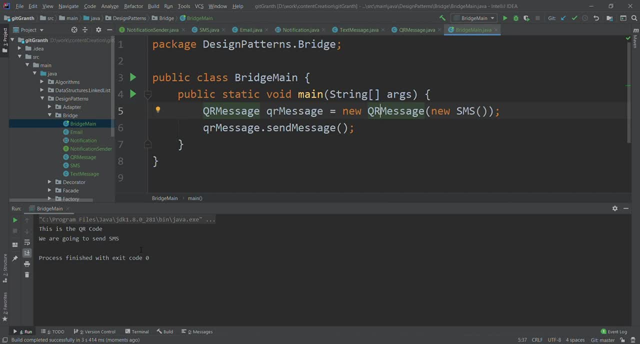 so we have to create n cross m kind of class and we have to create n cross m kind of class and that was the whole motto of using this notification service. so i hope you liked the explanation. do hit the like button comment. if you have any any understanding issue, just go back in.